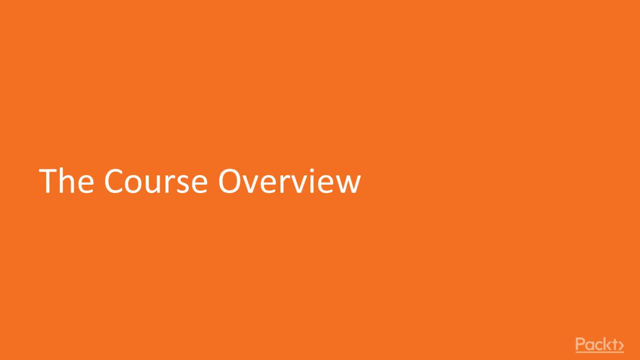 to analyzing data and the basics of statistics. This is an application-oriented course. The approach is going to be practical. The course discusses the situations in which you would use each statistical technique, the assumptions made by the method, how to set up the analysis and how to interpret. 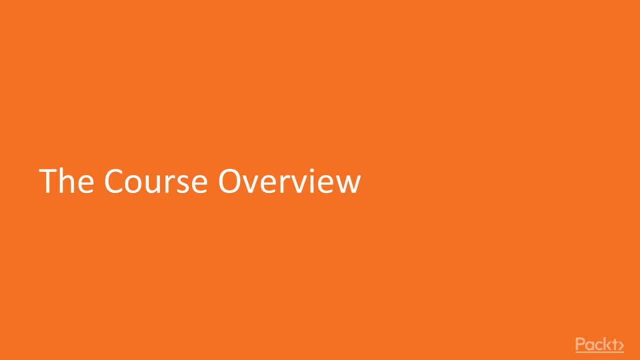 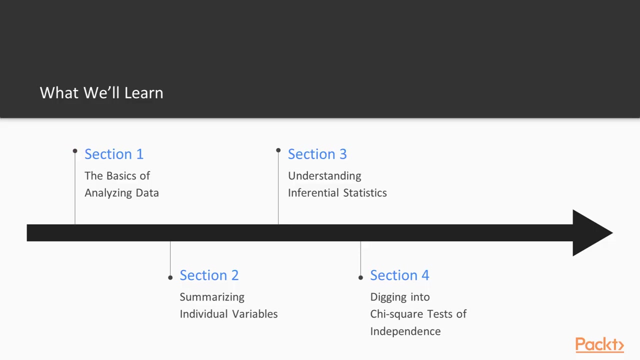 the results. No proofs will be derived, but rather the focus will be on the practical matters of data analysis in support of answering research questions. The first section of this course focuses on the steps to analyzing data and which summary statistics are relevant given the type of data that you are summarizing. 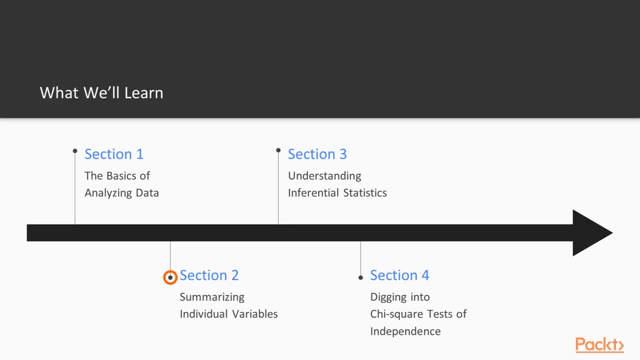 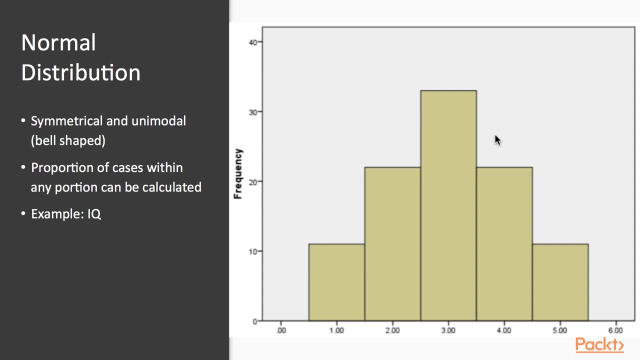 The second section of this course continues by focusing on summarizing individual variables and specifically addressing some of the reasons why users need to summarize variables. In this section, we will also illustrate several procedures, such as how to run and interpret frequencies and how to create various graphs. 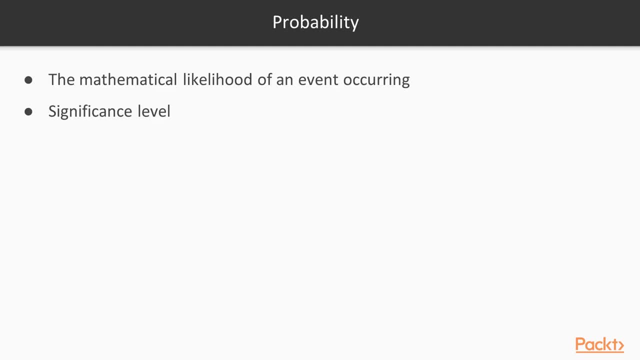 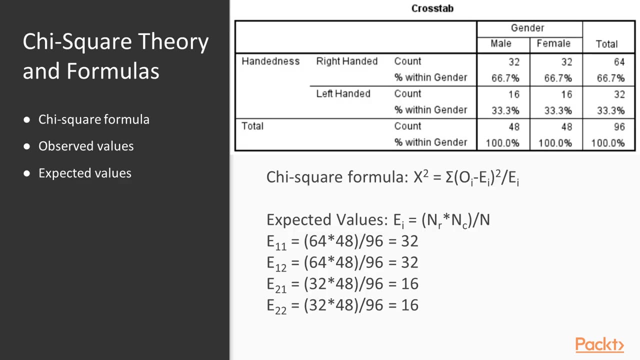 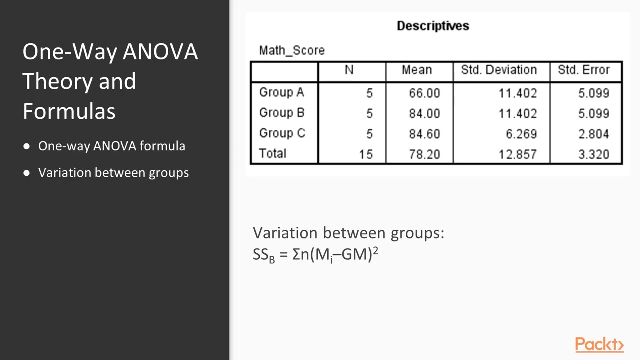 The third section introduces the idea of inferential statistics, probability and hypothesis testing. The rest of the sections show users how to perform and interpret results of basic statistical tests. We will talk about the chi-square test of independence, independent and paired samples tests one-way, ANOVA and its post hoc tests and bivariate correlations. 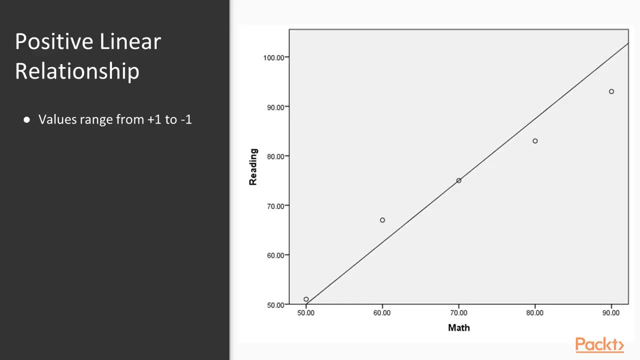 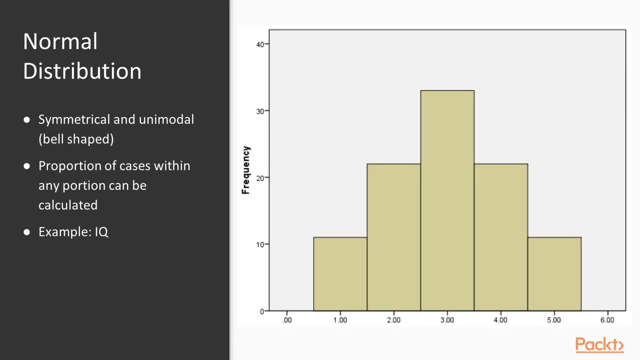 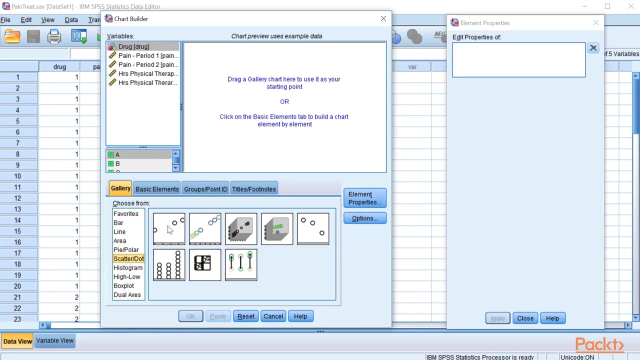 We're also going to show different graphical displays. So not only will you be able to run these different statistical tests, but you will also be able to create graphs that can accompany the results of your statistical tests, so you can visually show your audience what it is that they're seeing. So you'll learn how to create things like cluster bar. 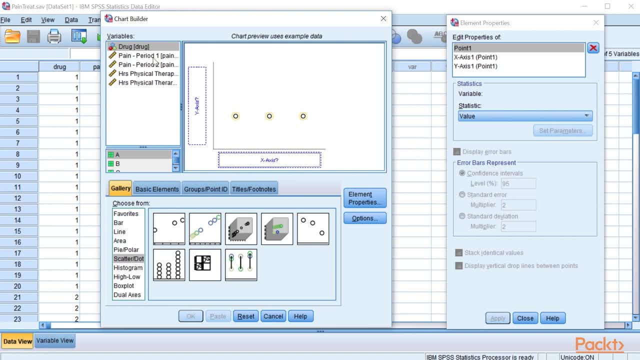 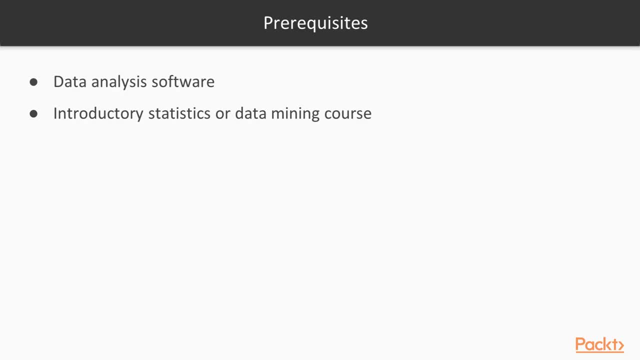 charts, error bar charts and scatter plots. Users will learn when to use these different techniques, how to set up the different analyses and how to interpret the results. Now this course is suitable for developers or anyone entering the field of data science who needs an introduction in analyzing data, as it covers the basics of statistics. This 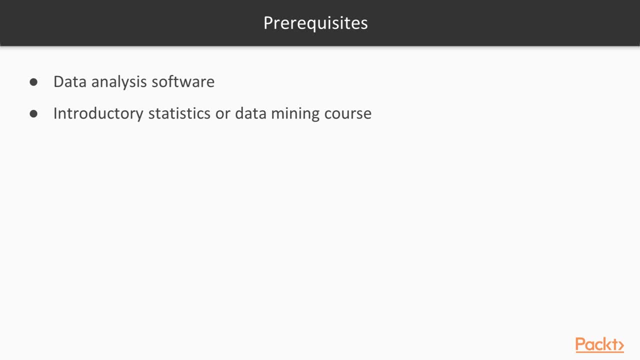 is an ideal course for those in data analytics, data management, data developers, data warehousers, data consultants, business analytics, business intelligence, statisticians, information security, information center finance, marketing and data mining- across all industries and sectors. 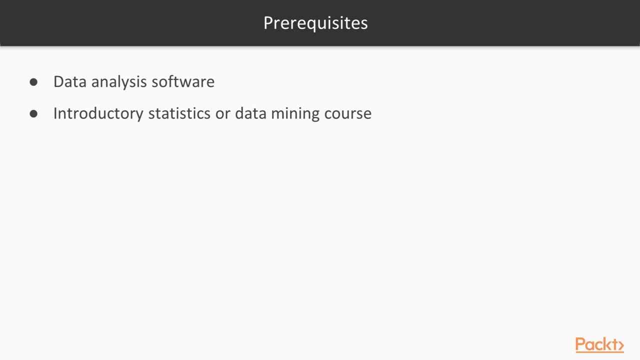 This course introduces students to the basics of data science, data analytics and scatter plots. Students do not need to be experienced in analyzing data, however. an introductory statistics or data mining course would be helpful. Here we're only going to take a short amount of time discussing different techniques, but